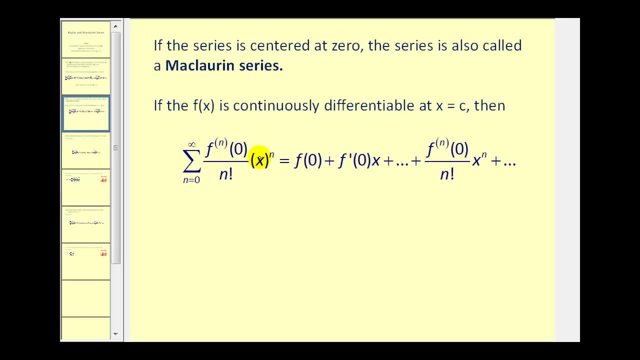 So we'll always have the nth derivative evaluated at 0. And instead of having x minus c to the nth power, we'll just have x. Let's go ahead and take a look at a couple of examples. Here we want to determine the Maclaurin series for f of x equals sine x. 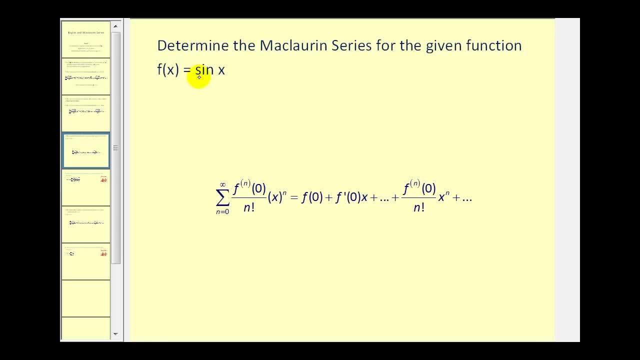 So again, here's the formula. What we're going to have to do is start with the original function and then find the first four or five derivatives of this function. Evaluate the derivatives at x equals 0,, since it's a Maclaurin series. 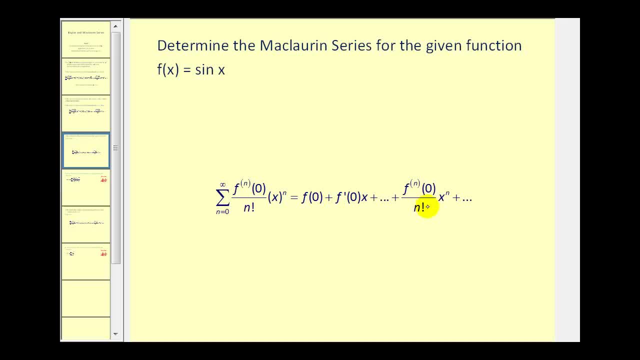 And then see if we can make a formula for the pattern we see as we find more and more terms. So f of x equals sine x. So the first derivative will equal cosine x. Second derivative will equal negative sine x. The third derivative would be: 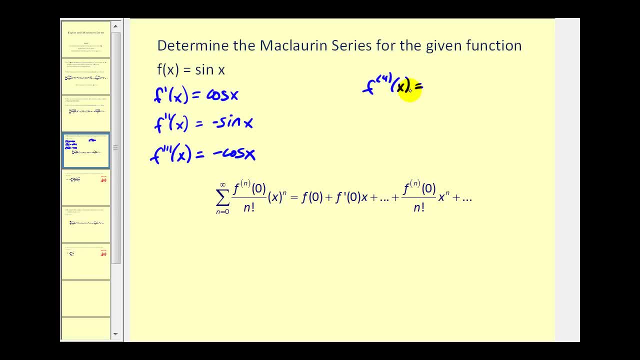 negative cosine x. The fourth derivative would be positive sine x. And let's find one more. The fifth derivative would be equal to cosine x. Now we'll go back and evaluate all of these at x equals 0.. So f of 0. 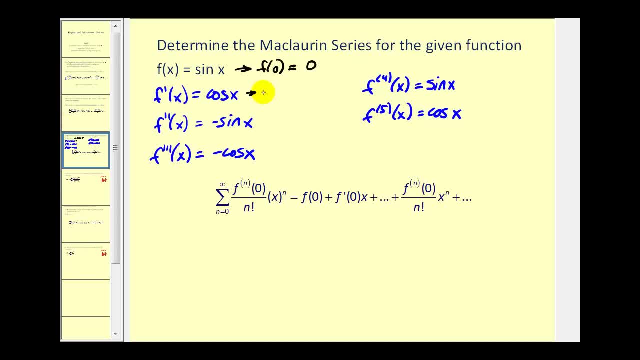 would be sine 0, which is 0.. f prime of 0 would be equal to cosine 0 or 1.. f double prime of 0 would be 0. again, The third derivative at 0 would be negative 1.. 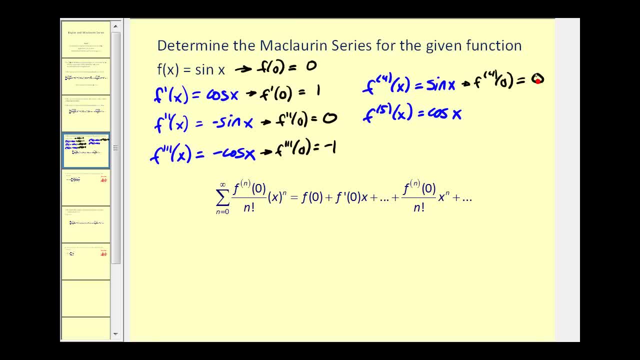 And then the fourth derivative at 0 would be 0.. And then the fifth derivative at 0 would be equal to 1 again. Now let's go ahead and find the first six terms of this Maclaurin series. So the first term is just f of 0, which is 0. 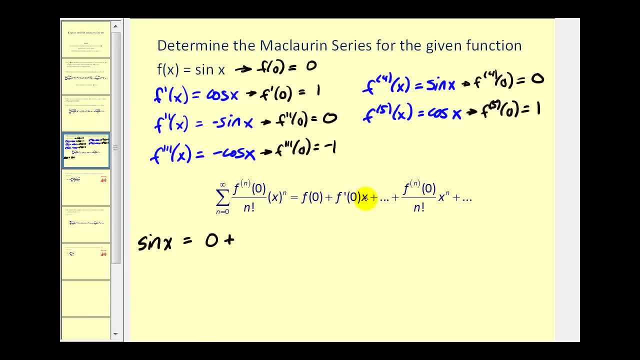 Plus the first derivative. if I, if I wrote it at zero times x, Well, that'll be one times x plus now we'll have the second derivative. if I wrote it at zero, that would be zero divided by n factorial, which is two factorial. 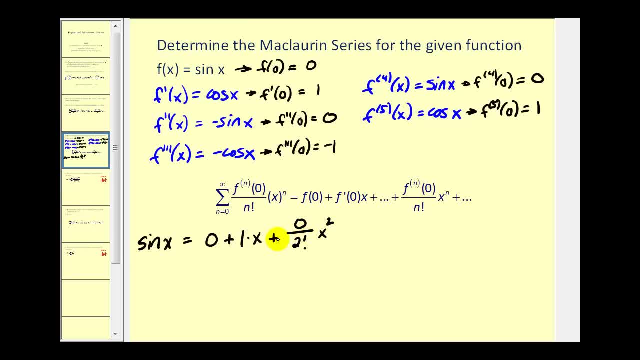 times x to the second. This term is equal to zero, but it is nice to see the pattern Plus the third derivative. if I wrote it at zero, that would be negative. one divided by n factorial times three: factorial times x to the third. 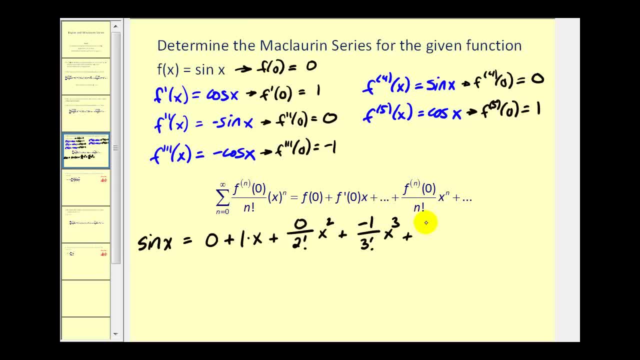 plus. the fourth derivative at zero is zero divided by four factorial times x to the fourth, and then we'll go ahead and find one more term that'll be plus. the fifth derivative at zero would be one divided by five factorial. 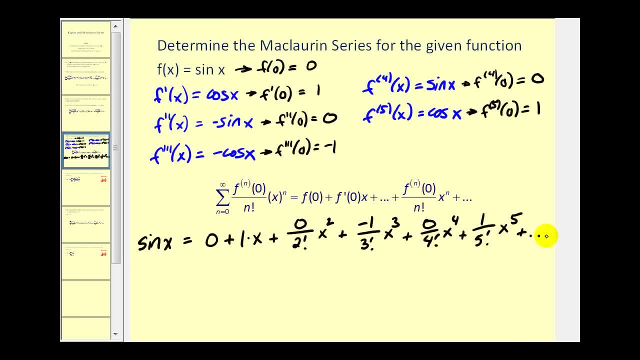 times x to the fifth, And of course, this continues. Let's go ahead and simplify this and see if we can discover the pattern to write the formula for the Maclaurin series. Well, this term is zero. this term is zero. 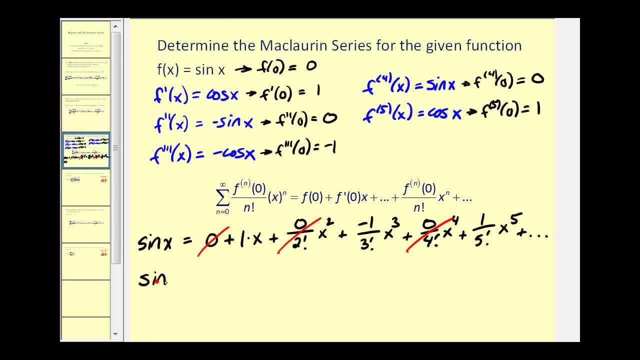 and this term is zero. So we have: sine x is equal to x, and then, instead of writing plus a negative one over three factorial, we'll write minus one over three factorial. x to the third, plus and one over five factorial. 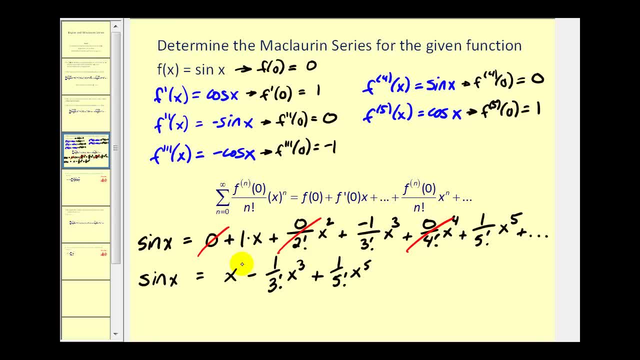 times x to the fifth. Here you can probably see the pattern. Notice that we have odd exponents on x and we also have odd factorials in the denominator as well as alternating signs. So the next term would be minus one over seven factorial x to the seventh. 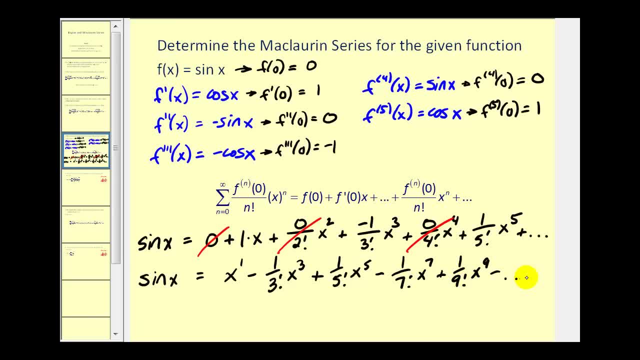 plus one over nine, factorial x to the ninth, and so on. So we have: sine: x equals the summation from n. equals zero to infinity of now. notice we have alternating signs, which means we'll have a factor of negative, one to the nth. 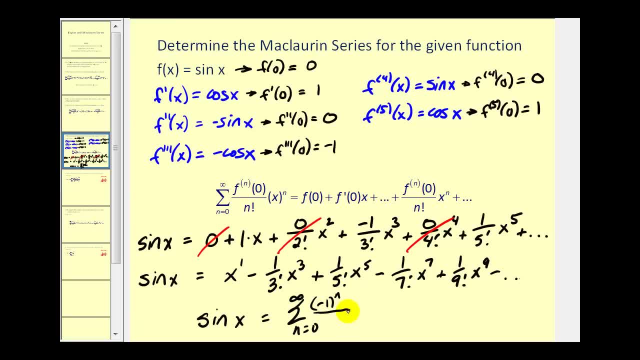 Our denominator is one factorial, three factorial, five factorial, So we'll have two n plus one factorial. and then we also have x raised to an odd power, So we have x to the two n plus one. Now we know this is true when x is equal to zero. 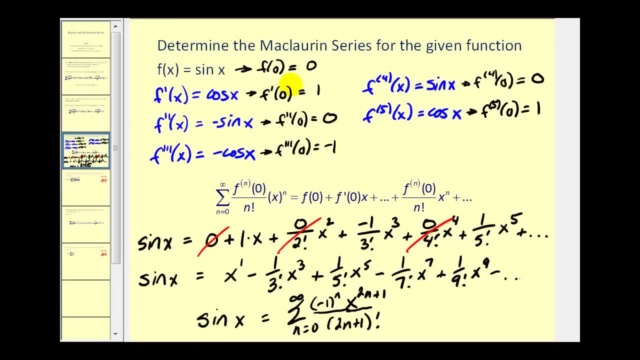 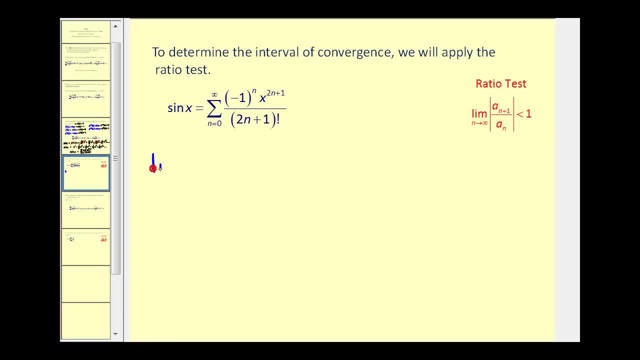 because that's where it's centered. Now let's take a look at the interval of convergence. Because of the factorials and the exponentials, we'll go ahead and apply the ratio test. So we'll take the limit as n approaches infinity, of a sub n plus one. so we'll replace n with n plus one. 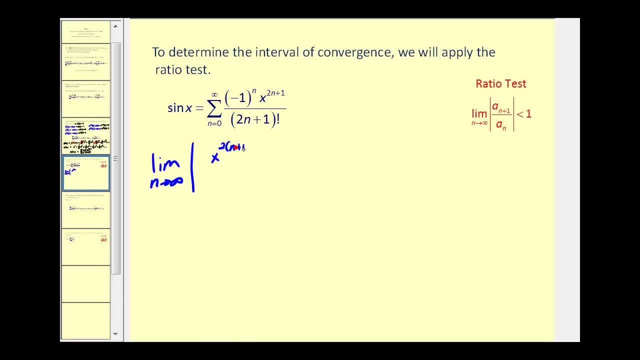 So we'll have x to the power of two times n plus one plus one all over. two times n plus one plus one factorial. Instead of dividing by a sub n, we're going to multiply by the reciprocal of a sub n. So we'll have two n plus one factorial all over. 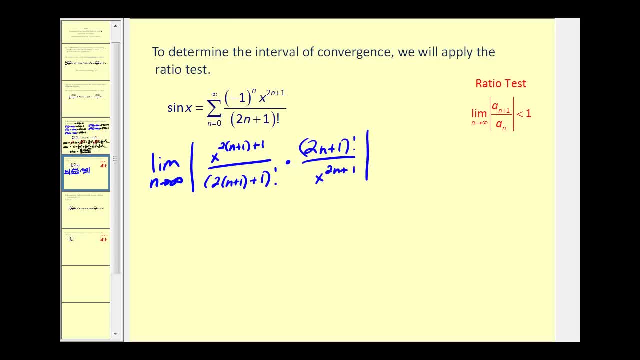 x to the two n plus one. Let's go ahead and take a look at this exponent. here We'd have two n plus two plus one, So this exponent is really two n plus three, And this is also two n plus three factorial. 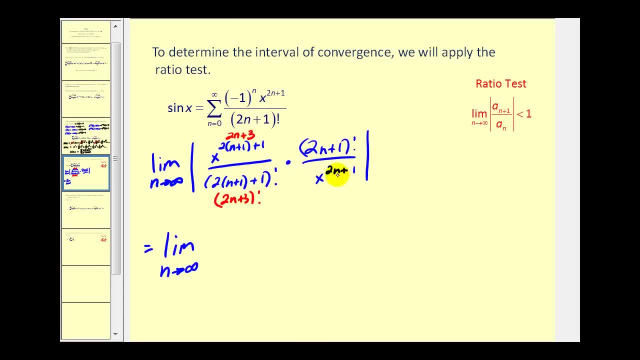 Now let's take a look at the factors of x. This has two n plus one factors of x and this has two n plus three factors of x. There are two more factors of x in the numerator: Two n plus three. factorial would be two n plus three. 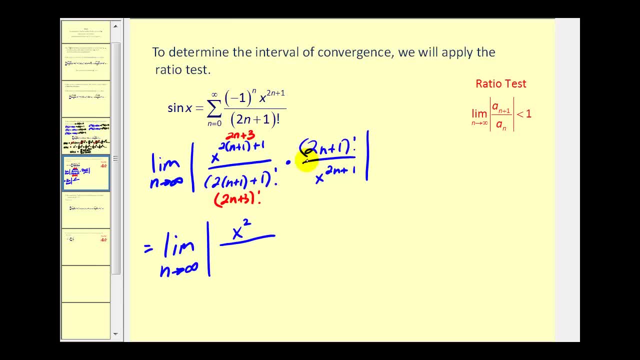 times two n plus two times two n plus one factorial. So we'll have a two n plus three and a two n plus two in the denominator. Now, as n approaches infinity, the denominator increases without bound. So this tells us: this element will always equal zero. 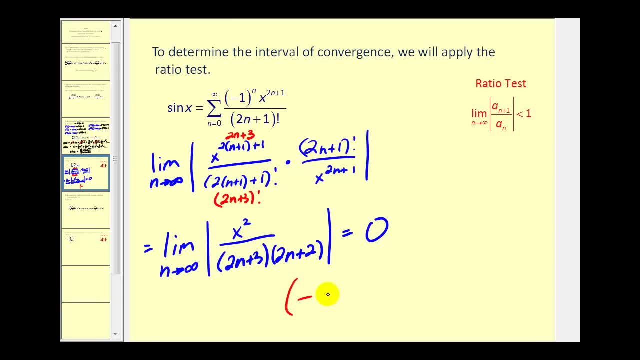 for any value of x. Therefore, the interval of convergence will be from negative infinity to positive infinity. Now let's go ahead and take a look at this Maclaurin series graphically. Here we have the graph of f of x equals cosine x, in blue. 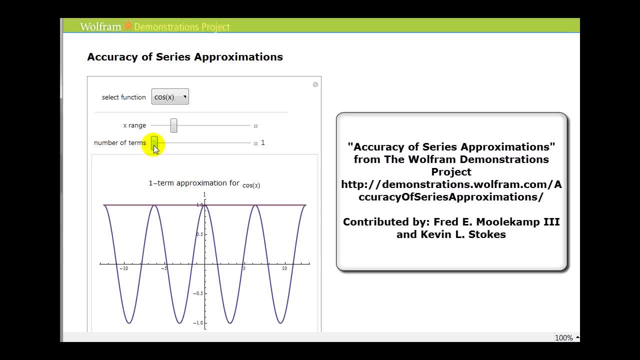 and then, in red, we're going to start adding terms to the Maclaurin series And, since the interval of convergence is from negative infinity to positive infinity, as we increase the number of terms, we're going to see the red function match perfectly with the blue function. 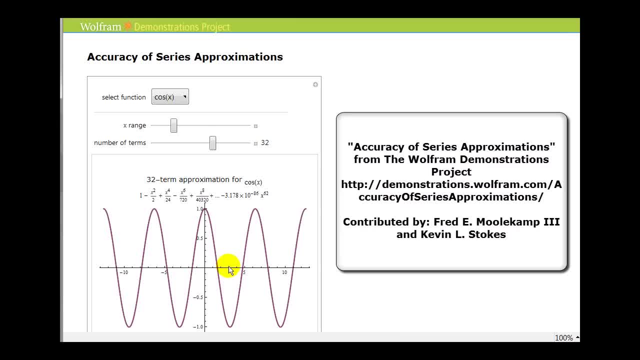 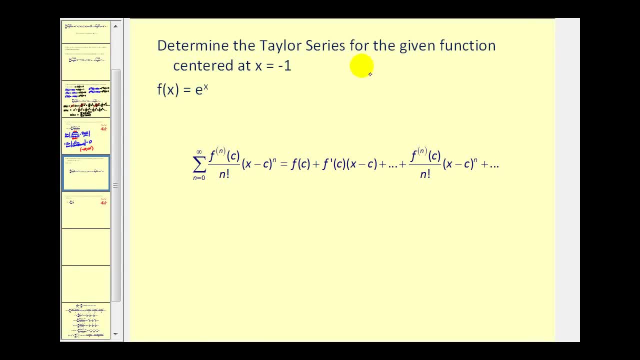 This is a nice way to show that the interval of convergence looks like it will be from negative infinity to positive infinity. Let's go and take a look at another example. We want to determine the Taylor series for f of x. equals e to the x. 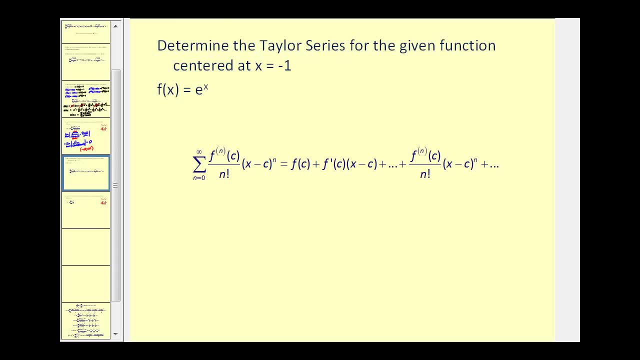 but now it's going to be centered at x equals negative one. So this tells us that c will equal negative one. therefore we'll have a binomial factor of x plus one. Another nice thing about f of x equals e to the x. 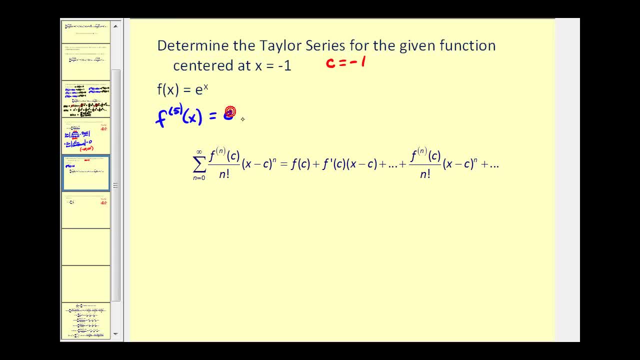 all of the derivatives of the function are also equal to e to the x. So with this information we can go ahead and start finding the first five or six terms of the Taylor series and then hopefully discover the pattern to write the formula for the infinite series. 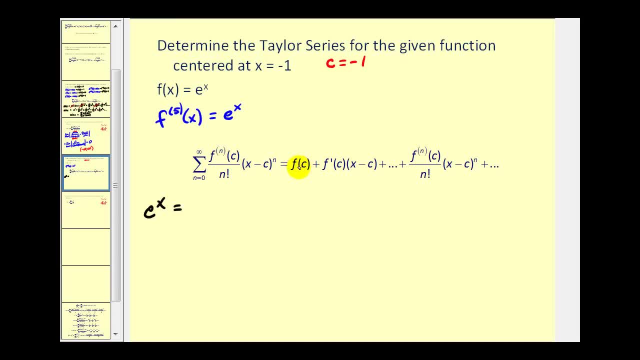 So we're going to have e to the x. it's going to equal the function value. when x is equal to negative one, that's going to be e to the negative one plus the first derivative evaluated at negative one times x plus one. 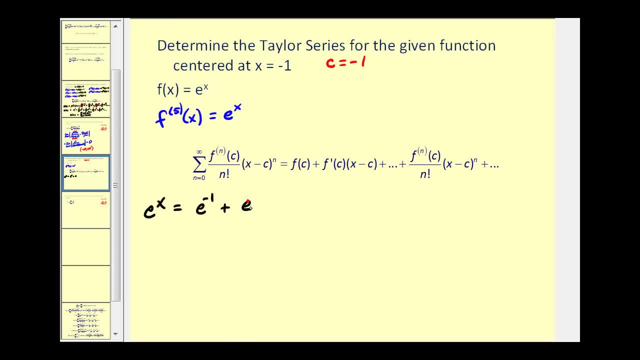 Well, the derivative is the same as the original function. so we'll have e to the negative one times x plus one to the first. plus now we'll have the second derivative evaluated at negative one. that'll still be e to the negative one. 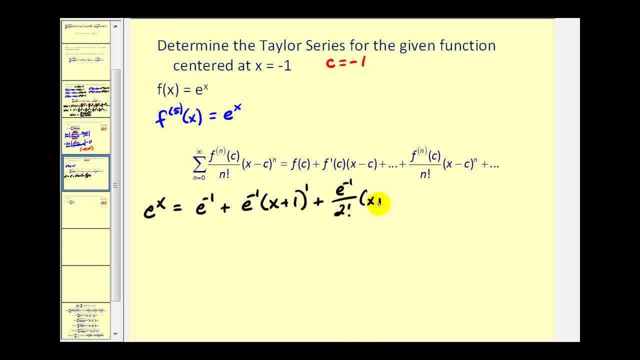 divided by two factorial times x plus one to the second, plus the third derivative evaluated at negative one is going to be e to the negative one, again divided by three factorial times x plus one to the third, and so on. So I think we have enough information here. 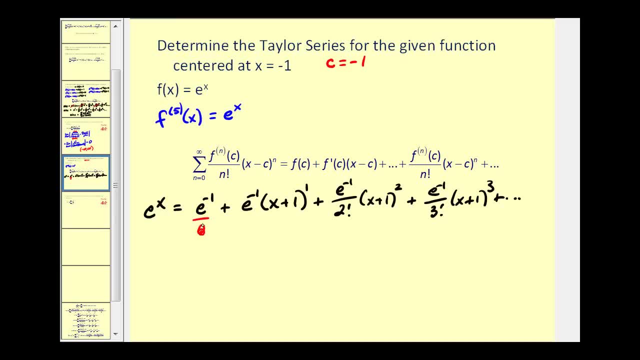 to see a pattern Again. remember this was divided by zero factorial and this was divided by one factorial. if that helps recognize the pattern, The first thing we should notice is that all of these terms have a factor of e to the negative one. 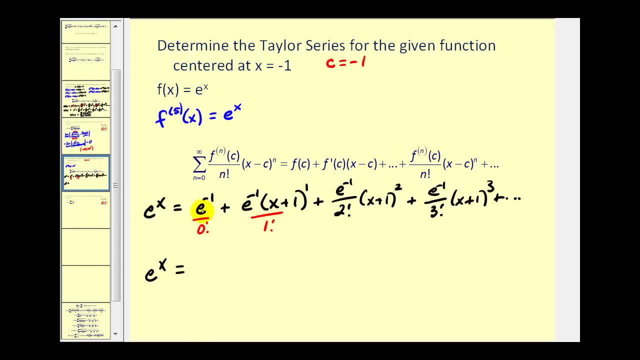 so we could factor that out of the summation and remember: e to the negative one is the same as one over e, So I have one over e times the summation from n equals zero to infinity. then we have these factors of x plus one, so we'll have x plus one to the nth. 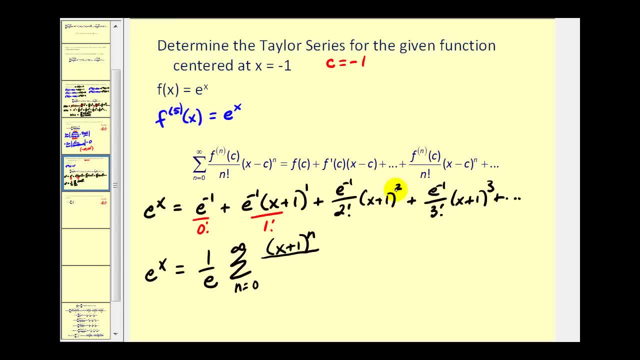 This would be x plus one to the zero, x plus one to the first, x plus one to the second, and so on, And then our denominator would be n factorial. Now, this is true when x is equal to negative one. so let's now determine the interval of convergence. 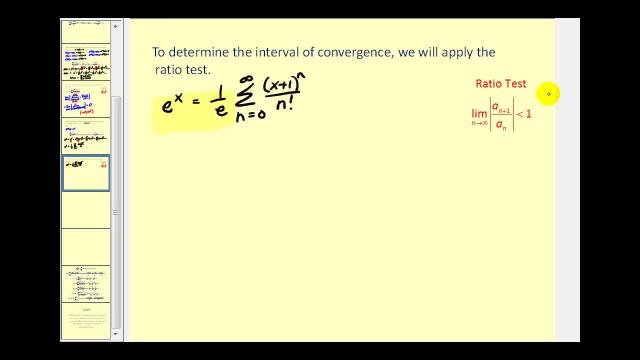 So to determine the interval of convergence of this, we'll go ahead and apply the ratio test, So we'll have x plus one to the n plus one power, divided by n plus one factorial, and then, instead of dividing by a sub n, we'll multiply by the reciprocal. again,